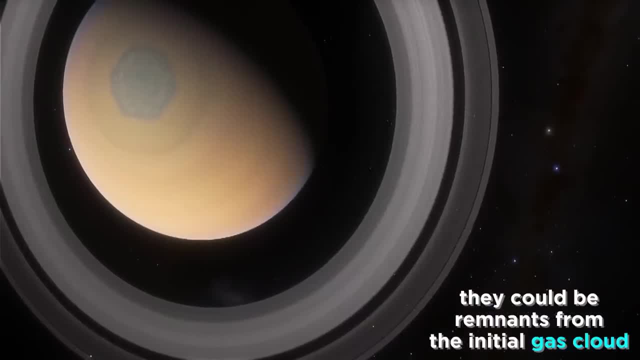 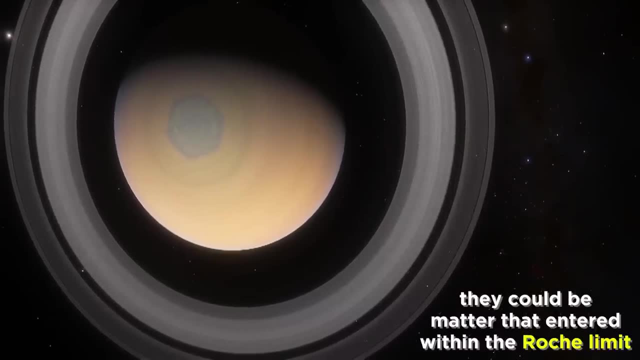 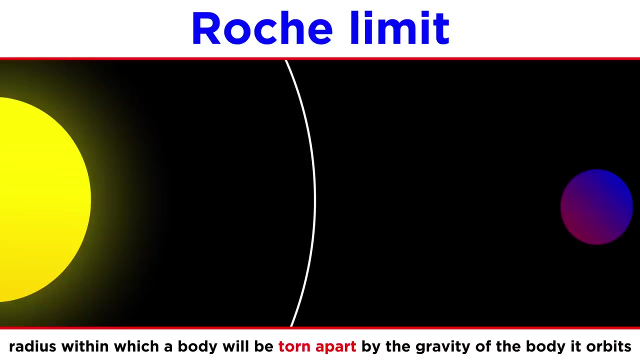 These are thought to be remnants of the cloud of gas and dust that initially formed the planet, though there are competing hypotheses that require the rings to be much younger. Some say the rings are comprised of debris from moons that enter the atmosphere. Some say they are entered within Saturn's roche limit, which, in this context, refers 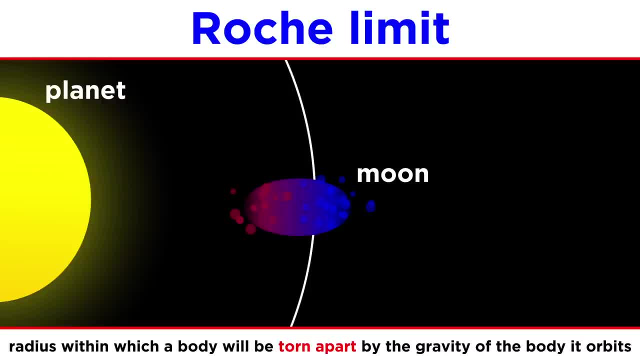 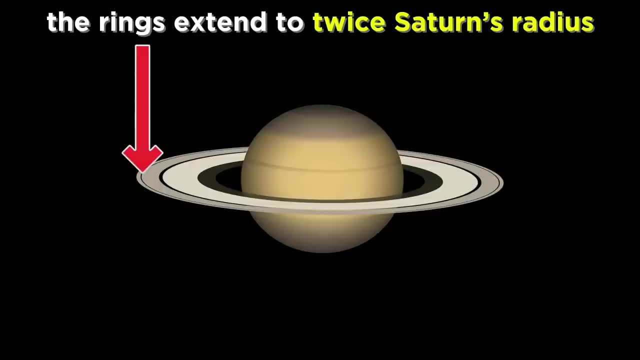 to the radius within which a moon will be torn apart by the gravity of its planet, Although, more generally, this term applies just as well to any smaller body orbiting a larger one, like a planet around a star. In any case, the rings extend out to more than twice the planet's radius, but are 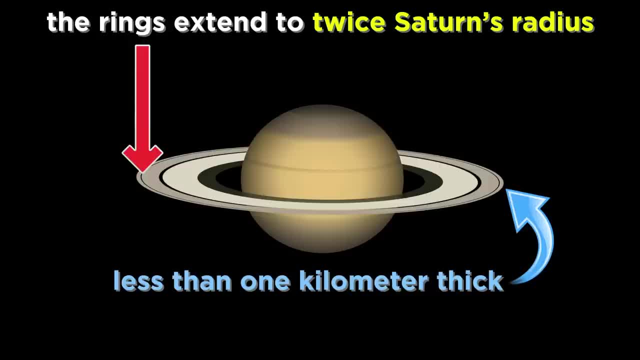 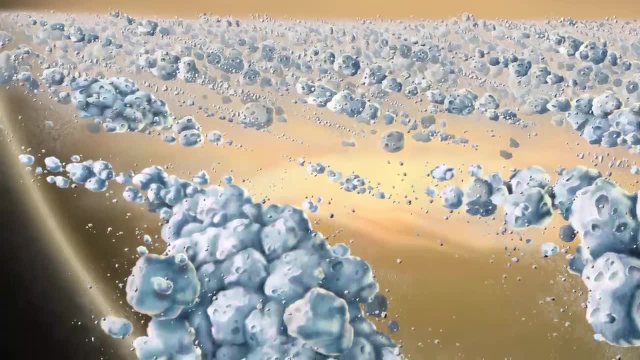 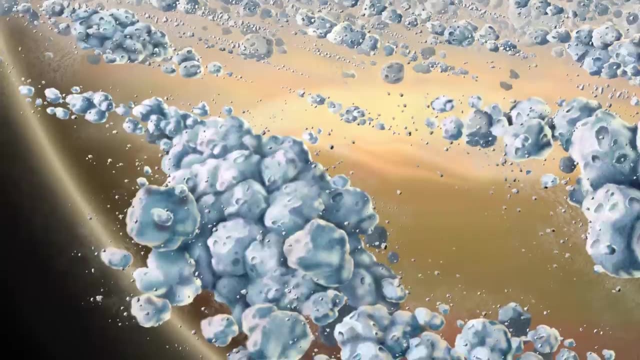 only a few hundred meters thick, which is incredibly thin by astronomical standards. Although they appear continuous from afar, they are actually just swarms of small icy particles ranging in size from a grain of sand to a school bus, orbiting at different velocities depending on their distance from the planet. 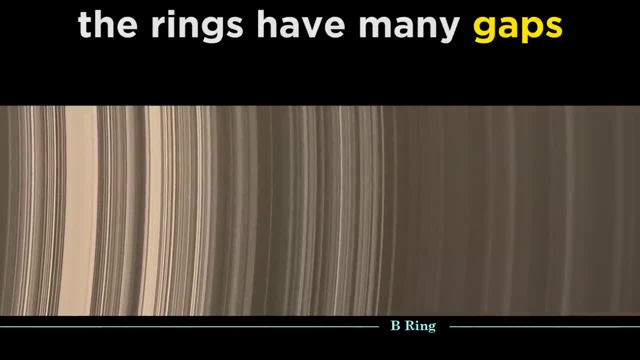 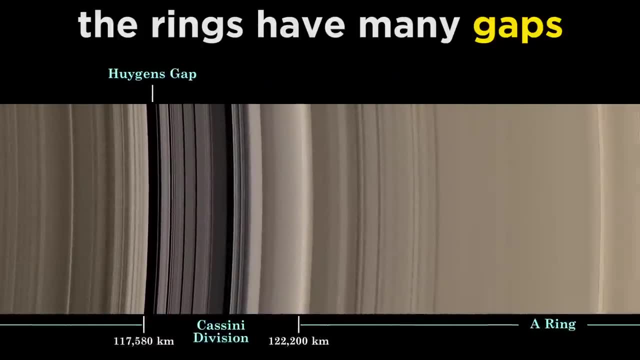 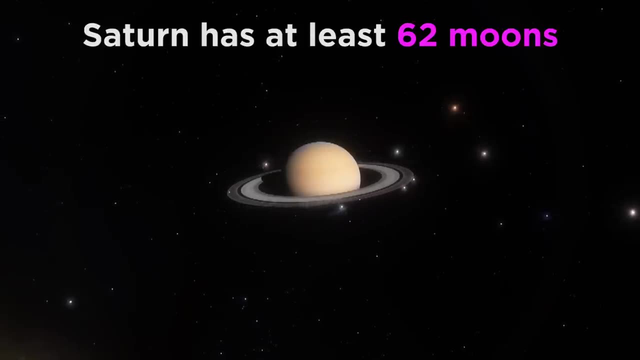 There are gaps in the ring system that have formed due to complex gravitational interactions amongst the particles, as well as some of the more closely neighboring moons. Speaking of moons, Saturn has lots of them, just like Jupiter does, so Saturn looks like yet another mini solar system within the solar system. 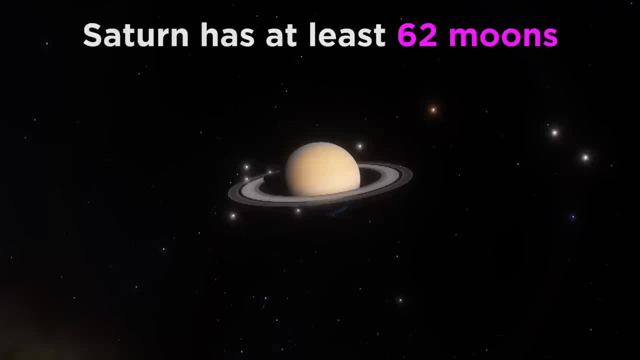 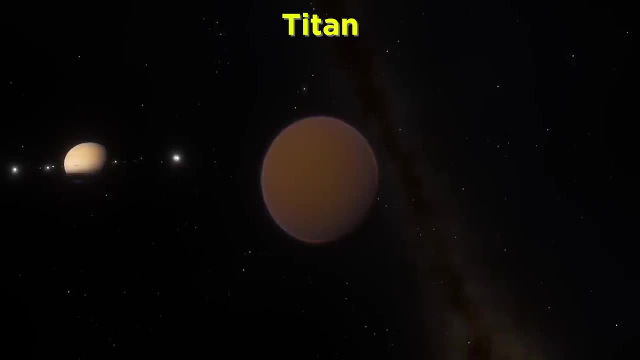 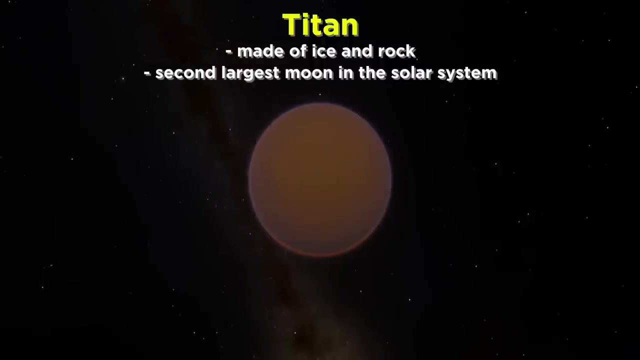 There are at least 62 of them orbiting roughly within the equatorial plane, and most of them have names derived from Greek mythology. By far the largest of these moons is called Titan. made of ice and rock, It is the second largest moon in the solar system after Jupiter's Ganymede and also 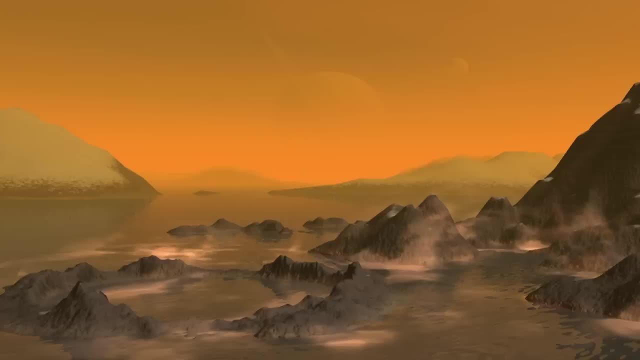 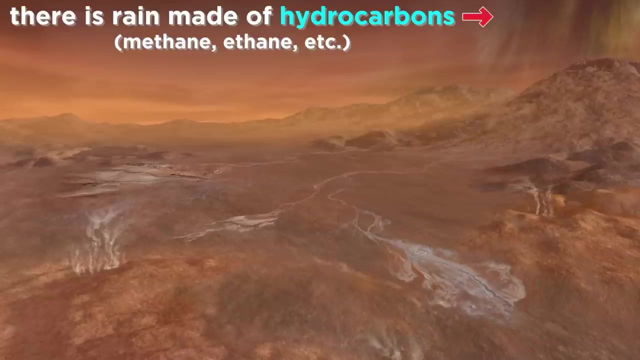 slightly larger than the planet Mercury. It is relatively far from Saturn and is thus rather cold, able to maintain an atmosphere, being one of only two known moons to have one, and this atmosphere is composed largely of nitrogen. Clouds rain down liquid hydrocarbons like methane and ethane, making Titan the only 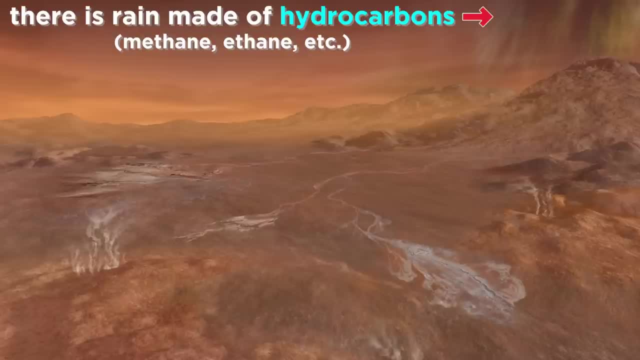 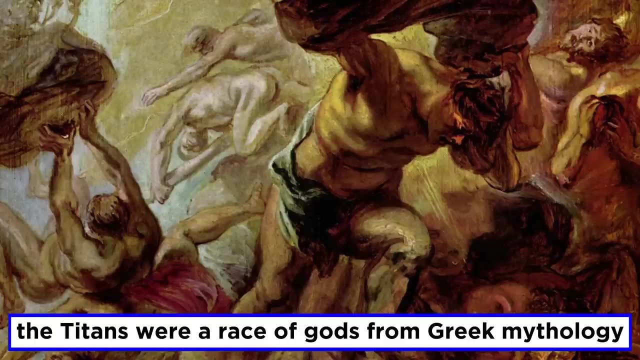 body in the solar system other than Earth to clearly have bodies of liquid on its surface. The Titans were the race of the moon. There are thousands of Greek gods directly descended from the first primordial gods and for this reason Saturn's largest moons have names taken from these Titans.